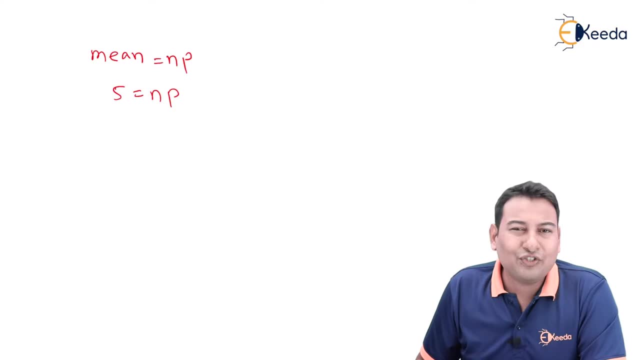 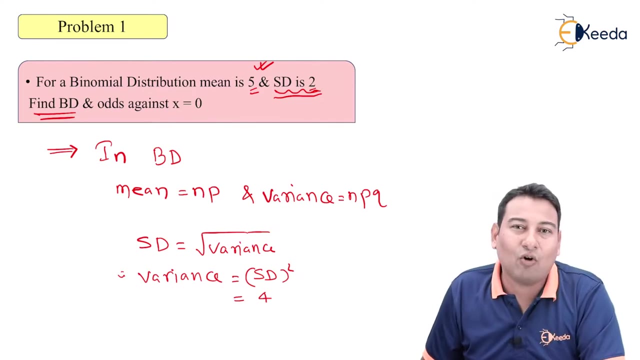 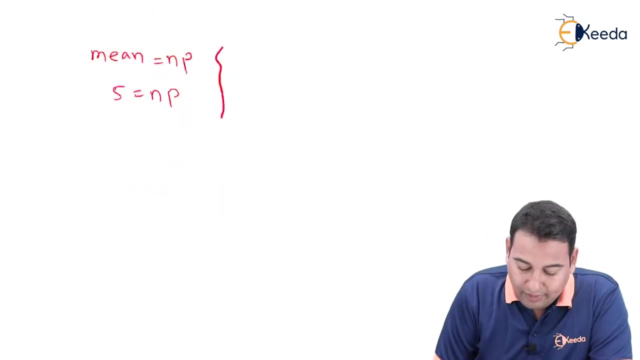 which is equal to np. Friends tell me for finding binomial distribution which is asked: what are the three terms that I want? n, p, nq. My aim is to get these three values- n, p, n, q, and variance formula is. 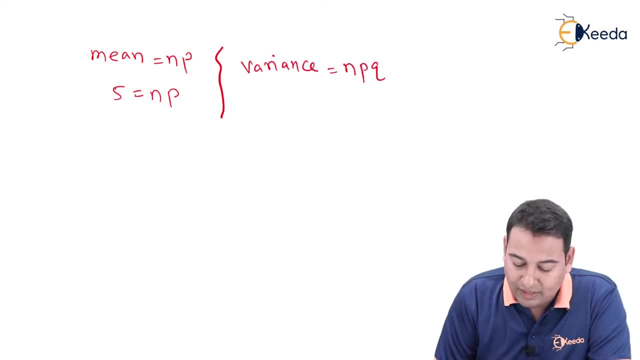 n p q Variance. we got it as 4, n p q. We need to simplify these two equations and we will try to get the value of n p n q. This np can be replaced by 5.. See, here you can replace this. Therefore, 4 is equal to. 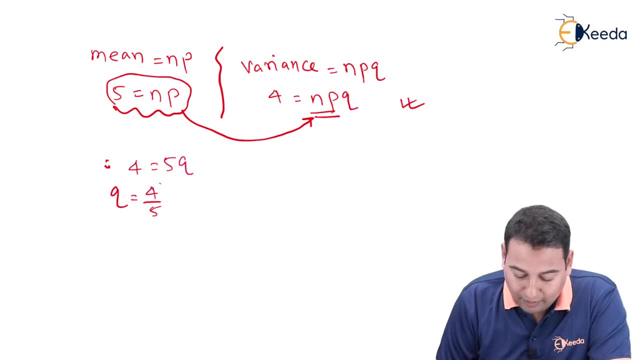 5q. q is equal to 4 by 5.. Out of three terms, we got first term, q. Also, we know, in case of binomial distribution, p plus q is equal to 1.. p is equal to 1 minus q. q is 4 by 5.. 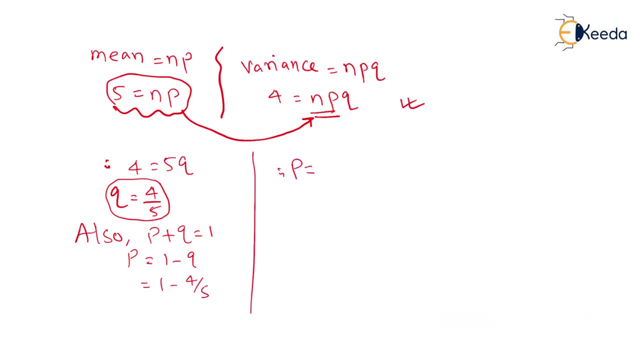 Therefore, P is equal to 1 by 5.. We are ready with P, We are ready with Q. What else N is needed? Mean is equal to NP. Mean is 5.. N is unknown. P is 1 by 5.. Cross multiply N is equal to 25.. 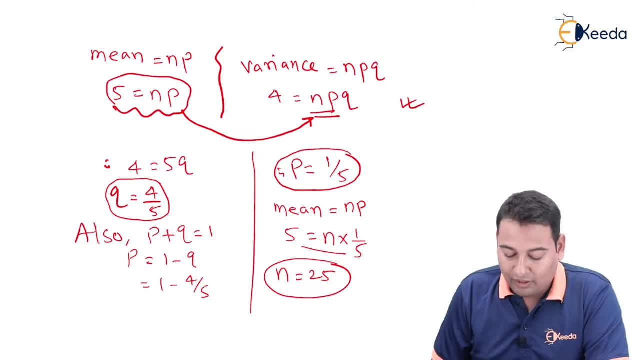 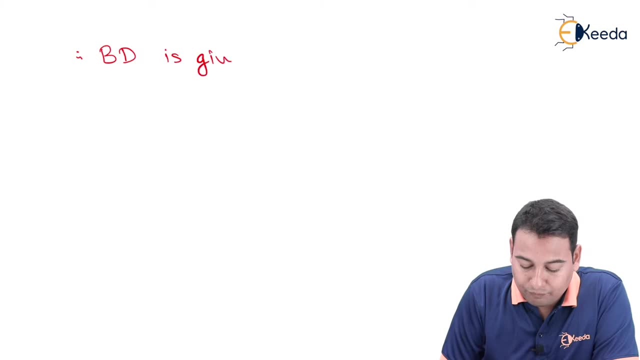 3 terms we need, and we got it: NP and Q. Therefore, binomial distribution is given by: yes. what is the formula? X equal to X, NCX, P raised to X, Q raised to N minus X. Let us put the values in the formula: N we got is 25.. C, X is not known, P. 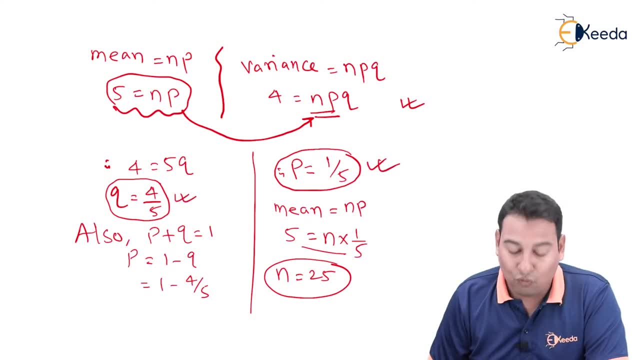 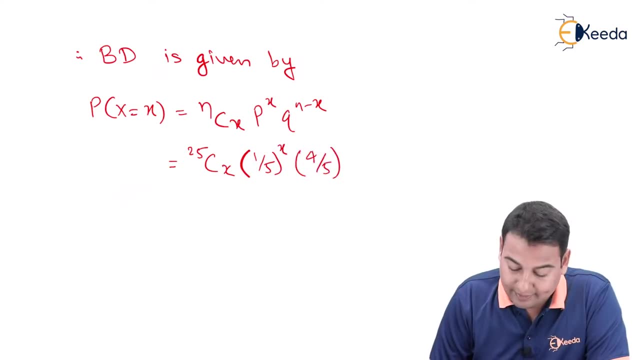 P is 1 by 5 and Q is 4 by 5.. 1 by 5 raised to X, 4 by 5 raised to N minus X, N is 25.. This is the probability distribution. So we got the answer for the first part of the question. 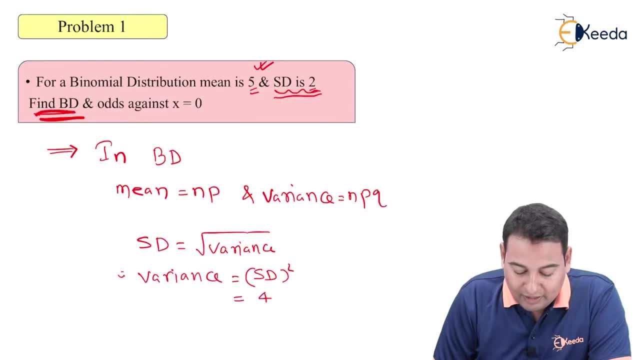 Let us discuss what is asked. First part is find binomial distribution. We got it and it is asked: Odds against X equal to 0.. Now remember: odds against X equal to 0 means 1 minus probability at X equal to 0..